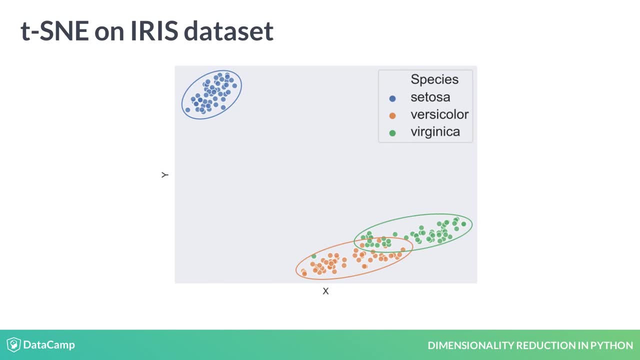 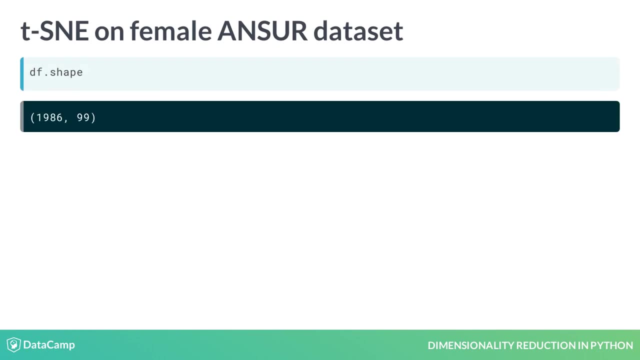 However, the IRIS dataset only has four dimensions to start with, so let's try this on a more challenging dataset. Our ANSER female body measurements dataset has 99 dimensions. Before we apply T-SNE, we're going to remove all non-numeric columns from the dataset. 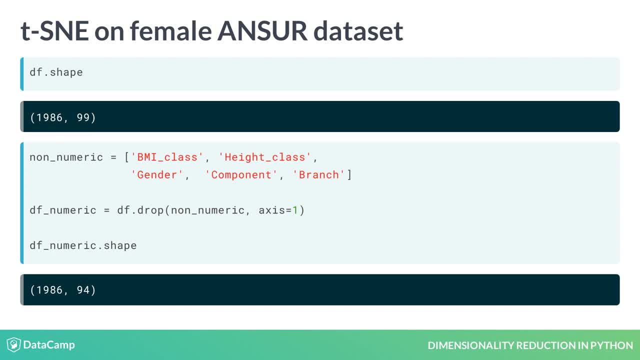 by passing a list with the data set. We're going to change the unwanted column names to the Pandas DataFrame drop method T-SNE doesn't work with non-numeric data as such. We could use a little trick like one-hot encoding to get around this, but we're using a different approach here. 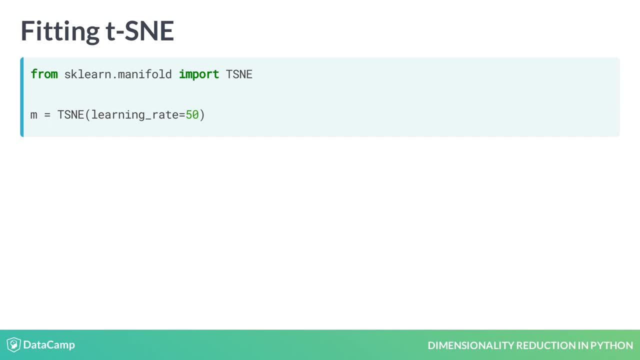 We'll create a T-SNE model with learning rate 50. While fitting to the dataset, T-SNE will try different configurations and evaluate these with an internal cost function. High learning rates will cause the algorithm to be more adventurous, while low learning rates will cause it to be more conservative. 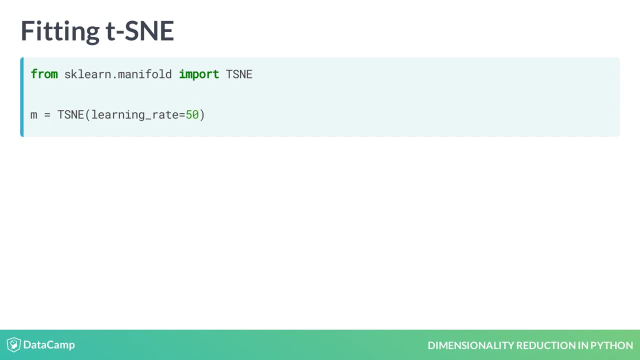 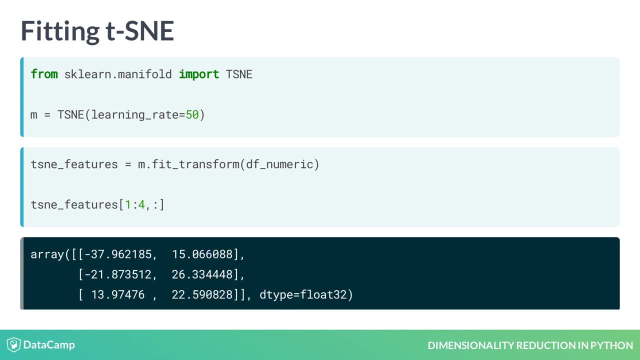 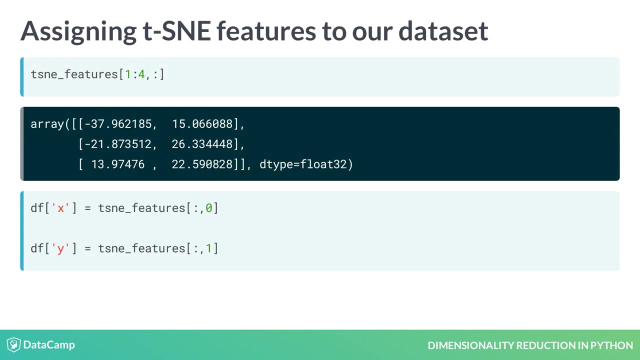 Usually, learning rates fall in the 10 to 1000 range. Next, we'll fit and transform the T-SNE model to our numeric dataset. This will project our high-dimensional dataset onto a NumPy array with two dimensions. We'll assign these two dimensions back to our original dataset, naming them X and Y. 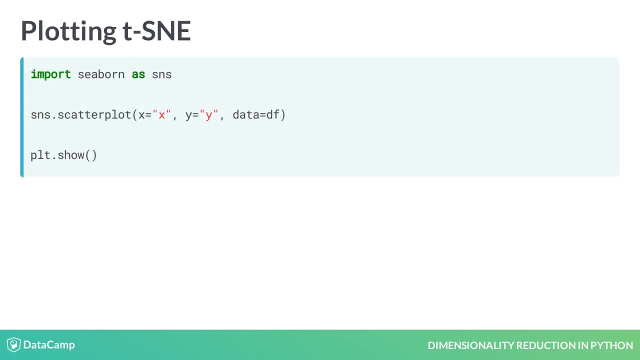 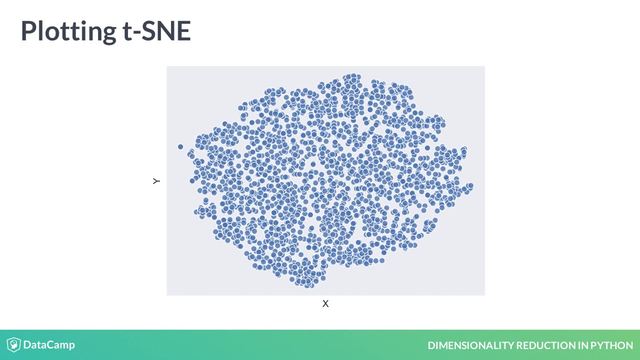 We can now start plotting this data using Seaborn's scatterplot method and the Y columns we just added. The resulting plot shows one big cluster, and in a sense, this could have been expected. There are no distinct groups of female body shapes, with little in between. 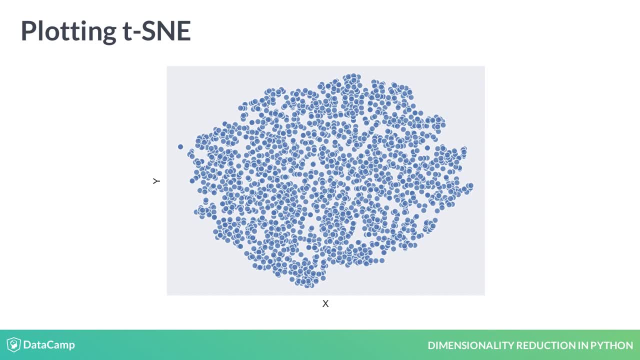 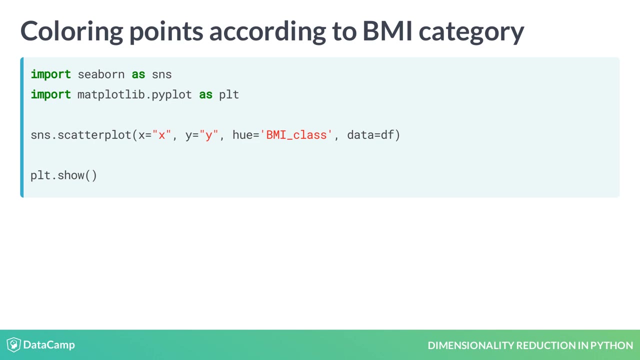 Instead, there's a more continuous distribution of body shapes and thus one big cluster. However, using the categorical features we excluded from the analysis, we can check if there are interesting structural patterns within this cluster. The Body Mass Index, or BMI, is a method to categorize people. 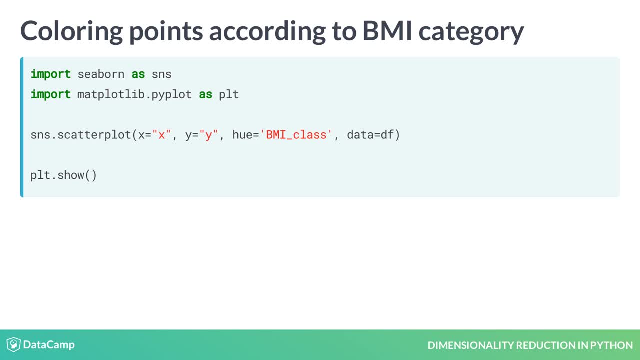 into weight groups, regardless of their height. I added the column BMI class to the dataset with the BMI category for every person. If we use this column name for the hue, which is the color of the Seaborn scatterplot, we'll be able to see that the weight class indeed shows an interesting pattern. 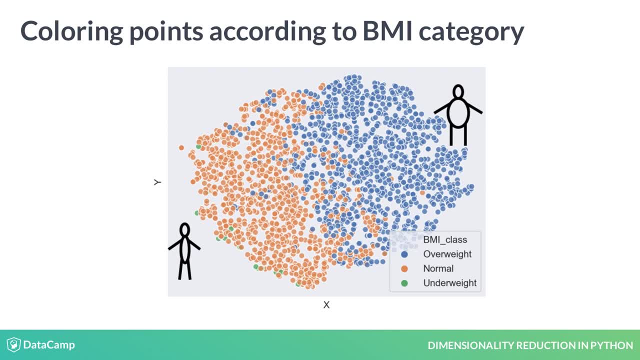 From the 90 plus features in the dataset T-SNE picked up that weight explains a lot of variance in the dataset and used that to spread out points along the X-axis, With underweight people on the left and overweight people on the right.